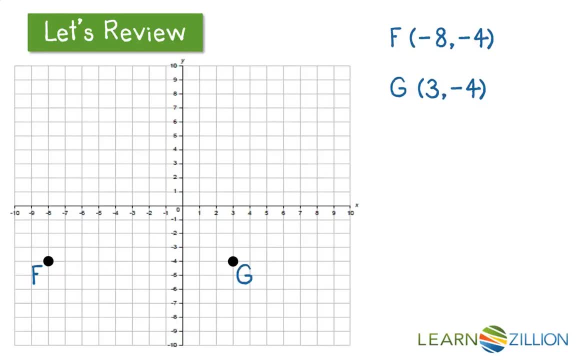 these two points are on the same line. Now we can find the distance between them by finding the absolute value of the difference of the X values. So we can find the absolute value of negative 8 minus 3, and that gives us an absolute value of negative 11.. Now it's important to remember that distance is always. 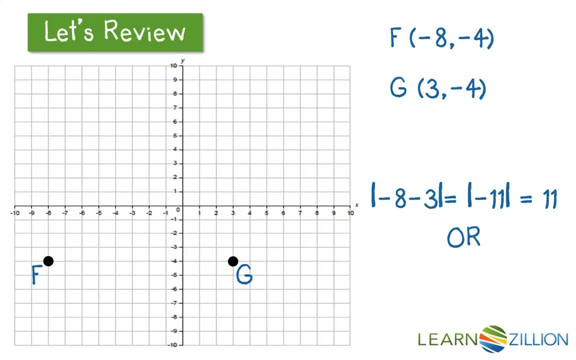 positive. That's why we use absolute value, because the absolute value of negative 11 is 11 units. Or we could say that the absolute value of the difference of 3 minus negative 8 gives us an absolute value of 11 or 11 units. So we can travel from F to G and 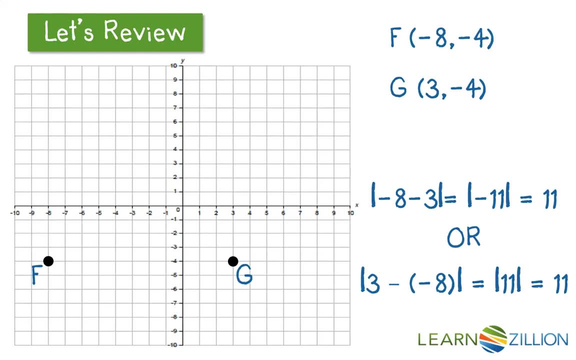 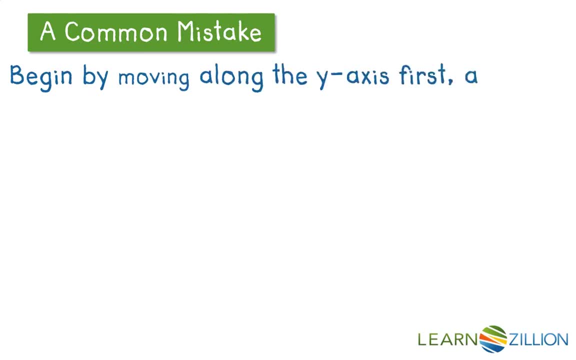 we have a distance of 11, or from G to F, and again we have a distance of 11.. A common mistake that I've seen many people make is that they begin by moving along the y-axis first and then along the x-axis when finding an ordered pair. 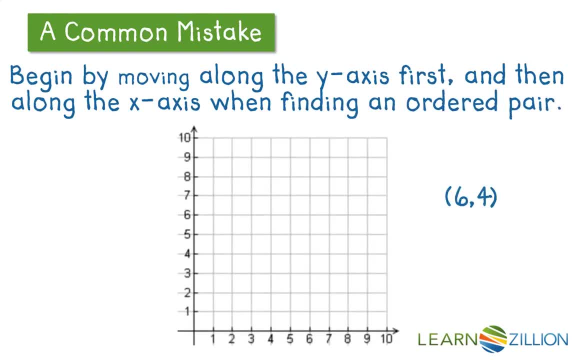 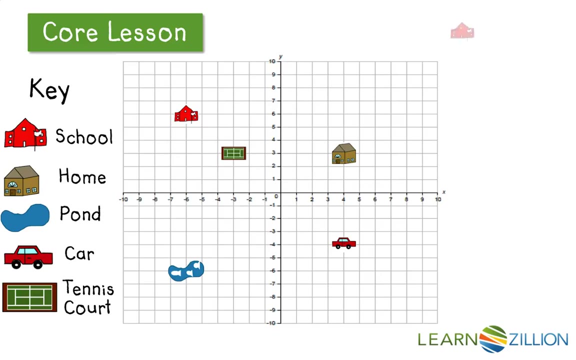 So in the case of ordered pair 6, 4, they would make the mistake of moving on the y-axis first and then on the x-axis. As we can see, that does not give us the correct location. Let's start by locating a few landmarks on our map. The school is located at negative 6, 6.. The 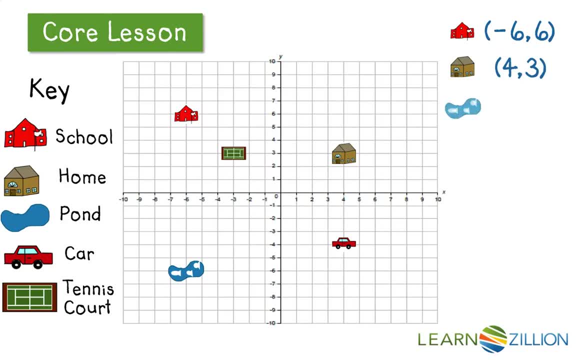 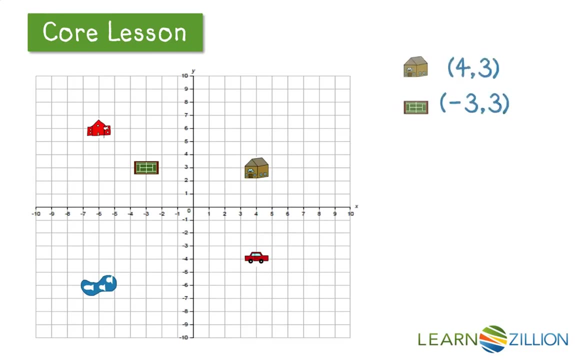 house is located at 4, 3.. The pond is located at negative 6, negative 6.. The car is at 4, negative 4 and the tennis courts are located at negative 3, 3.. What is the distance between the house and the tennis courts? 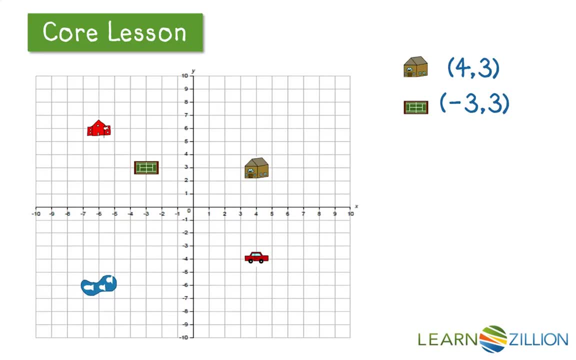 Now these two points share a y value, so we can find the distance by looking at the absolute value of the difference of the x values. So I can start at the house and I can find the absolute value of 4 minus negative 3, which gives me an. 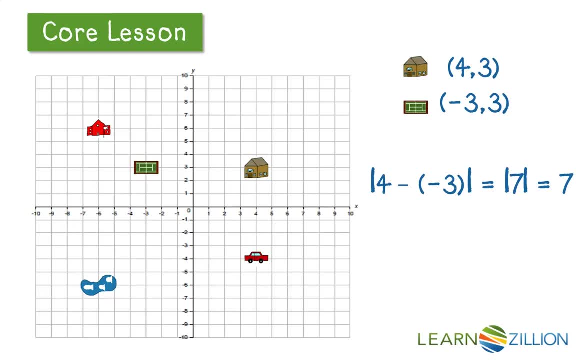 absolute value of 7.. I know that the distance from the house to the tennis courts is 7 units. If I was traveling from the tennis courts to the house, I could find the absolute value of the difference of negative 3 minus 4, which.